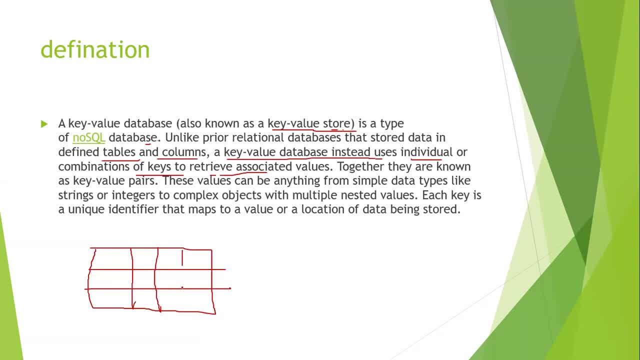 In this rows and columns. here you have student number right. Next you have name of the student and then we have marks of the student. Then we have like total or phone number of the student. Here these type of databases are called as relational databases. So the software. 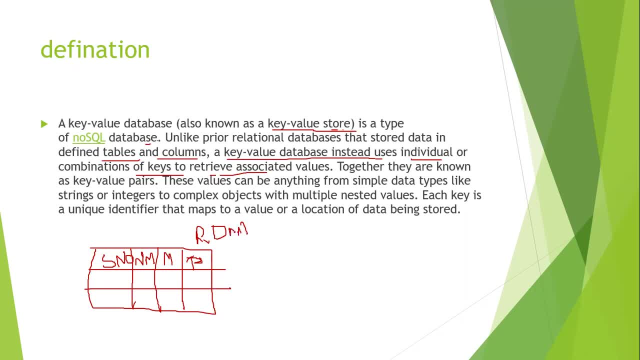 which is used to implement this is RDB- RDBMS- relational database management system. So this RDBMS uses structured query language to retrieve the data from the databases. So here here we have details, for example, But whereas this key value database, it should not contain the details of the students or 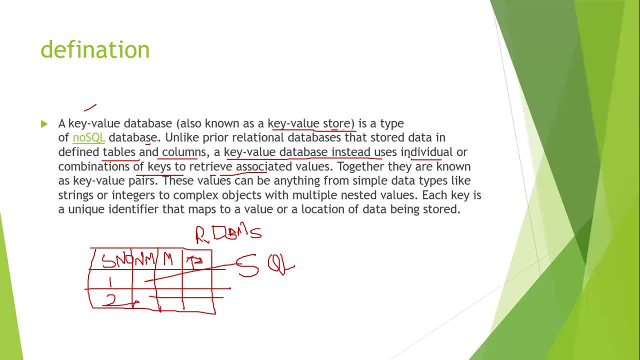 any record. What it has instead uses individual or combination of key value database, So it's just a combination of keys to retrieve the associated values, For example, this particular record right. This particular record is stored at a address A1. So this particular student. 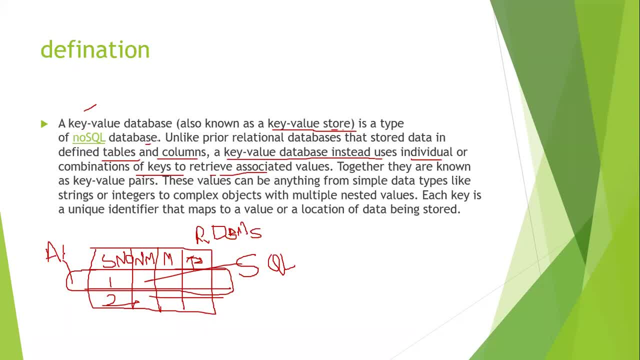 details are storing in a memory. The memory name is A1.. Then this key value database have keys and values. So the key one- consider key one- contains the values of students and students. So the key one- consider key one- contains the values of students and students. 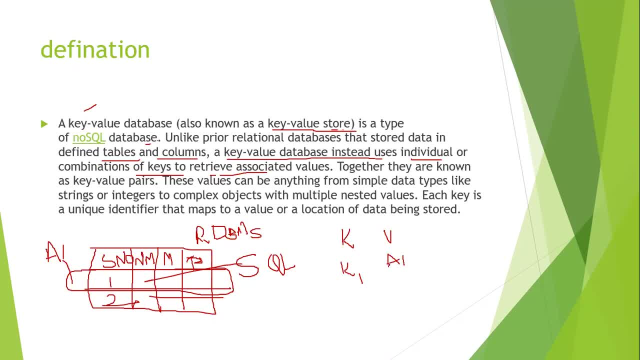 value as a1. that means this key 1 have the row a1. the row is presented in a memory cell instead of having record details. what we are doing we are storing the record in a particular location in the memory and that address we are writing in a key and value pair. now these values can be. 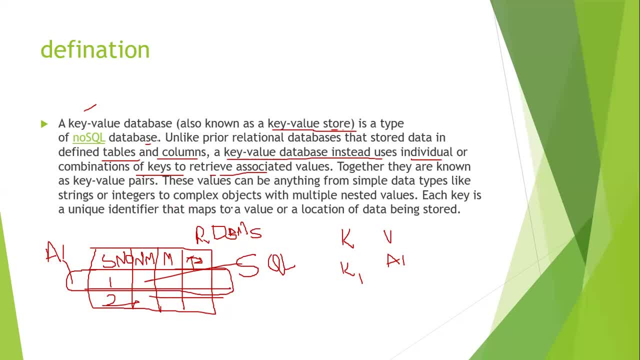 anything from simple data types like strings, integers, to complex objects with a multiple nested values. each key is unique identifier. that means what? what the keys you have here- k1, k2, k3, k4, all these are- must be these keys. values must be unique. they not be repeated. so if you know, 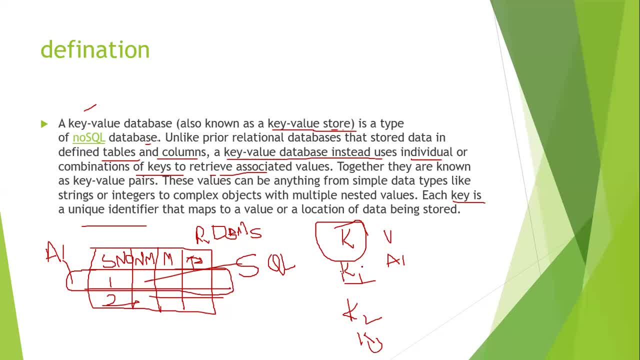 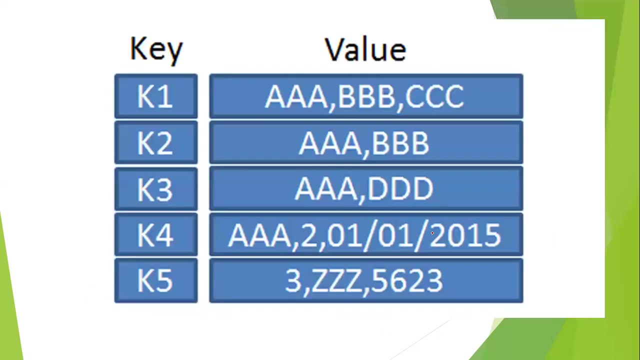 key 1. that means internally in the memory. this k1 is having the address of a1. so internally control goes to a1 memory location. in that memory location what details you have? we have student number one and the respective details of the particular student and this data will be getted to the data base. so here we'll see example. see here: k1, k2, k3, k4, k5. 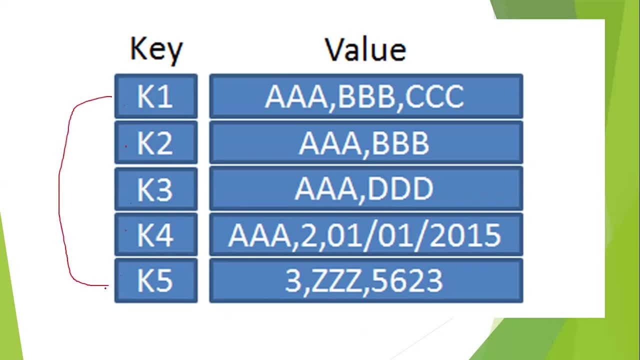 all these are what? all these are the different types of keys and these keys also unique. so values. so values are nothing but address locations. so a, a, b, b, b, c, c, c, all these are the different addresses of the memory blocks. if you are mapping k, so this k maps to. 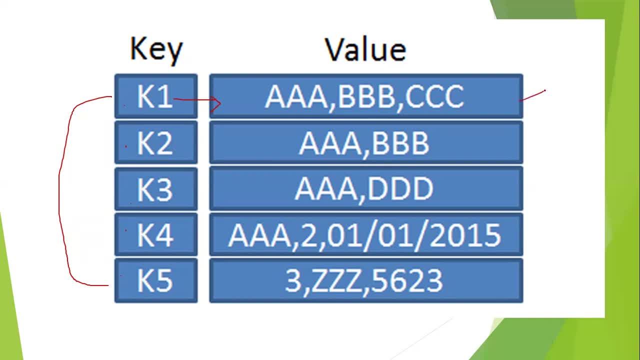 this three, then after from there what the details you want, whether you want a details or whether you want b details or whether you want c details. from there we can retrieve the data from the particular locations. so these values may be one or any combination of three. that means what? 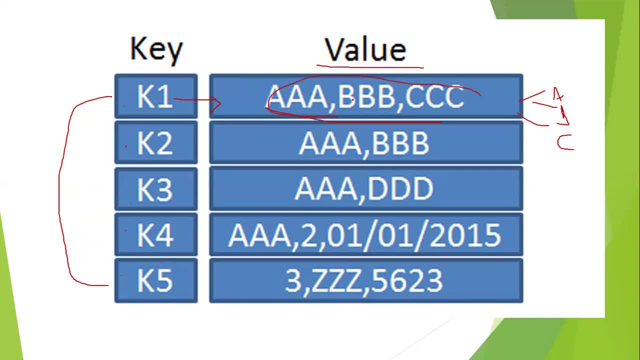 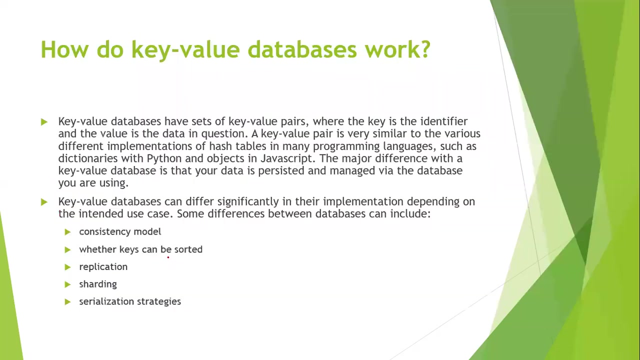 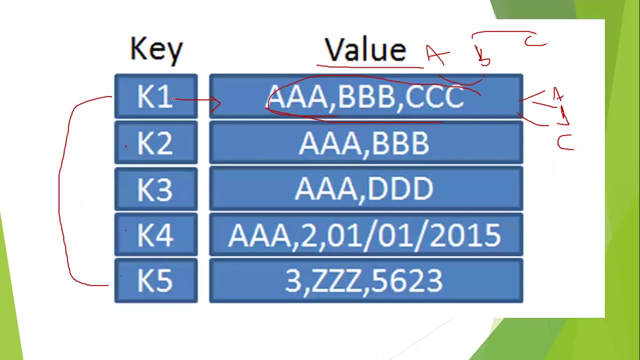 here keys are individually unique, but values are not unique. so that means value can be retrieved as a combination of any number of keys and rows, and but the keys must be unique, clear. so here, key value database, how it works. so how it works just now, only i explained you first. it will take the key and this key value. 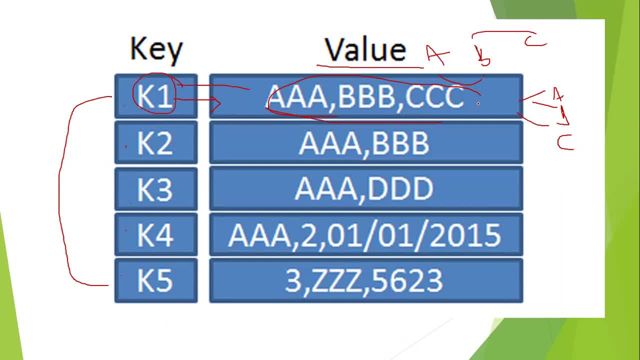 database have a sealedAB 3 for Which roles this you get only this is a simple trazor domain memory kind of central area, so it takes it 한곤 participier, which feature means you can have a 3D a little bit of every main collector and task team, not all you have. to do what? capacitors which says 코를 penaj wishlist. where is the block a? this three blocks are there. these three blocks are able. these, these blocks are blocks. this a, block a. this is a block b. this is block c Building. They are mapped and the date of these three tables they don't. these three memory blocks will be retrieved. throwsh servicio within the since six take the back a day out to the use. not see here. key manager databases have a safe. 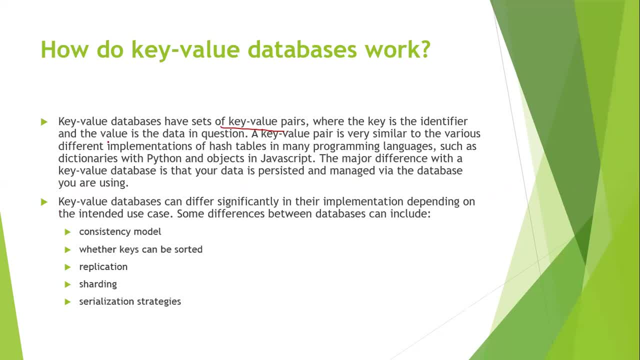 of key value pairs where the key is identifier and the value is in the data in the question. a key value pair is very similar to the various different implementations of hash tables in many programming languages. the major difference with the key value database is that your data is. 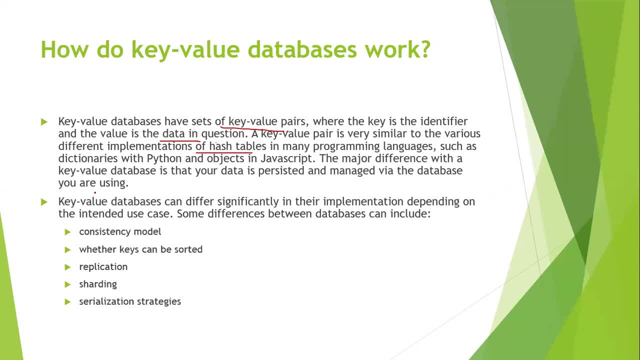 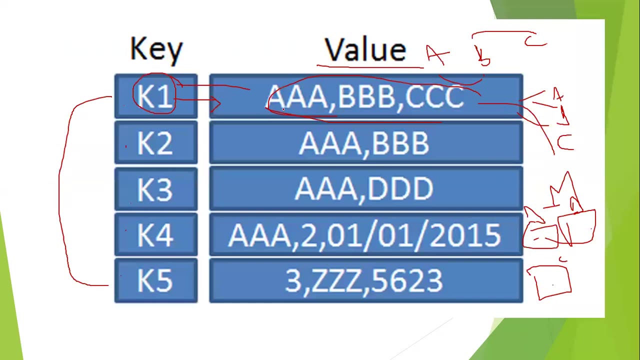 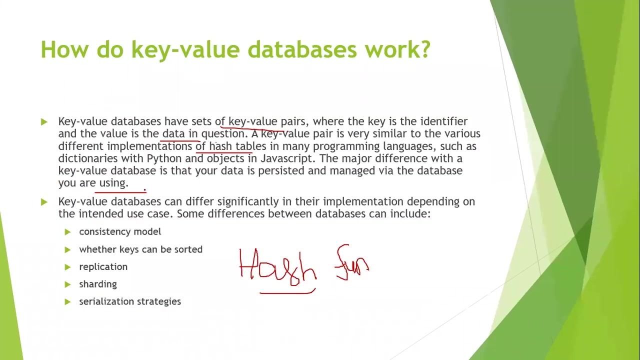 persisted and managed via database you are using, so by using hash function. so keys and values as well as the values. okay, so how to implement hash function will come to know in the later classes. key value database can differ significantly in the implementation depending upon the intended use case. that means: 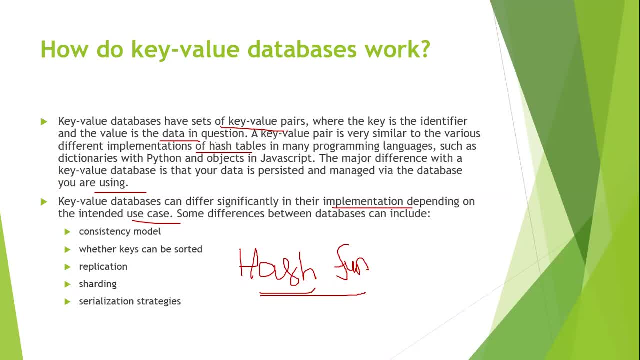 the key value database is not in the same format according to the user's choice, for example, iot application or government services application or online applications or any application based on the use case. that means the use case in which we use it, in which use case we should use the key. 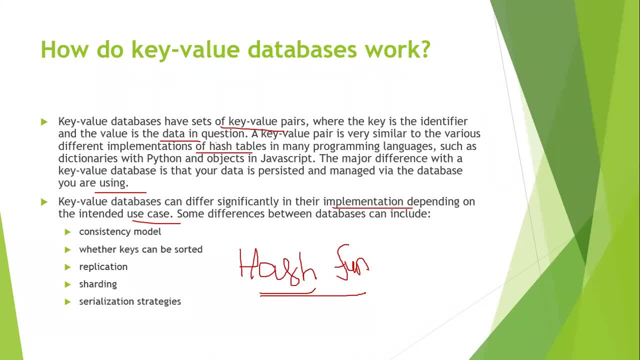 value database. according to that, we have to make variations. so some of the differences- differences between databases- can include consistency, model keys, replication, shareding and serialization strategies. so one database goes up and another data base has a lot of different data bases available. so we can find the most tabular skill between exactly this樓 and the others, based on 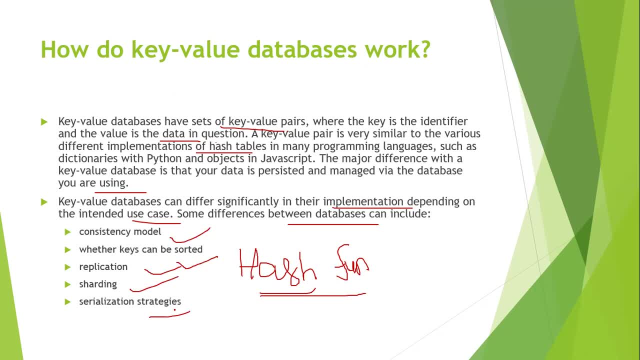 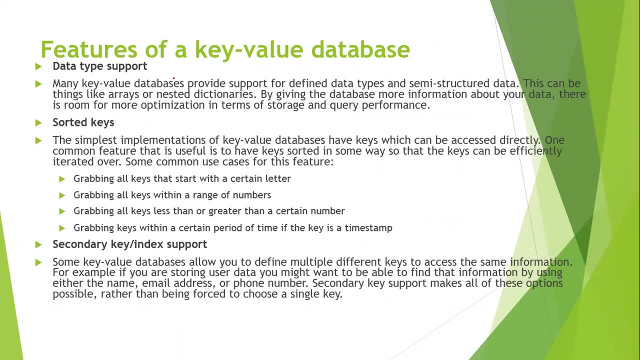 use case if need be. we can find the most tabular skill between. we can find the most tabular skill base, certain tabular skill reference and the other type of tabular has to be like whatever diversity among the five differences. next one is what features of key value database. so if you do one, first, data type. 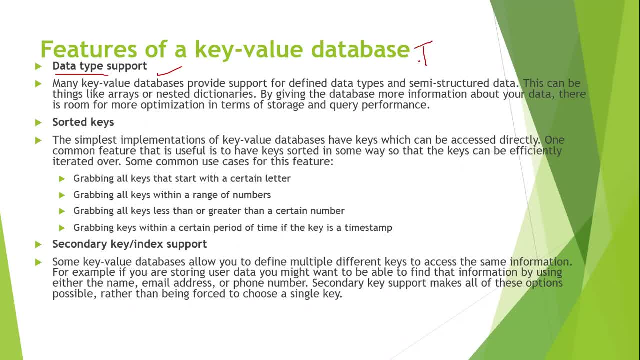 support. that means what it can store in data. so that means this numerical type data. it can store integer data like maps, data data, so then we will grabbed by the key values so the data so store, character type of data it can store and combination of special character type of data. 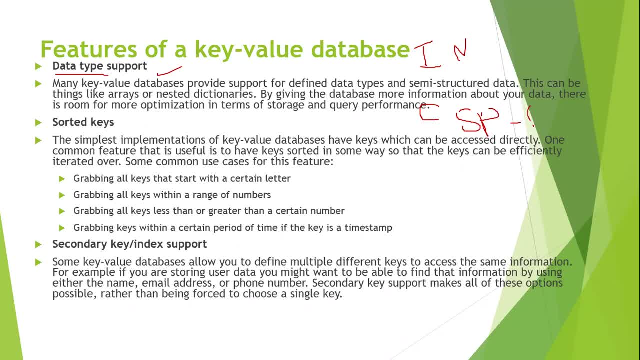 it can store underscore. it can store floating point data. it can store hexadecimal point of data it can store. so data type is nothing but type of data you are storing in a database. so semi-structured data and things like arrays, nested dictionaries, all the information will be stored in. 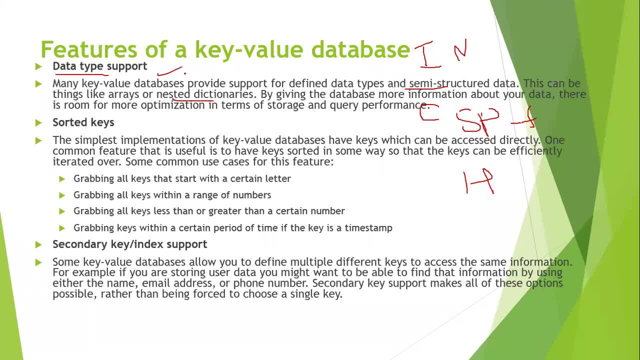 your database. that means any type of data can be stored in the key stored database next to sorted keys. so this is the main feature. you can see nothing but what. for example, k1, k2, k3, k4, like this, all keys are there. so all these keys are in what? in a sorted order. so what these are? 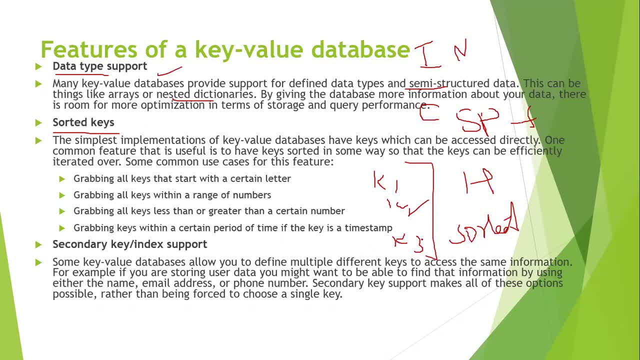 in sorted order. if the order is not there, you cannot easily access the data. for example, consider your book. okay, in your book you have index pages, right, all index pages are. for example, your book consists of one to hundred numbers, so 10 numbers one chapter, 10 numbers 10. 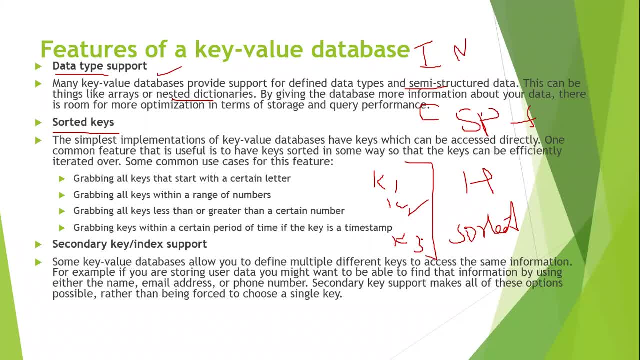 papers one chapter: 10 papers one chapter. if you want to search for a particular topic, just we go to index and we search the particular topic and we go to respected page number. so if the pages are not in a particular sorted order we cannot search very easy. 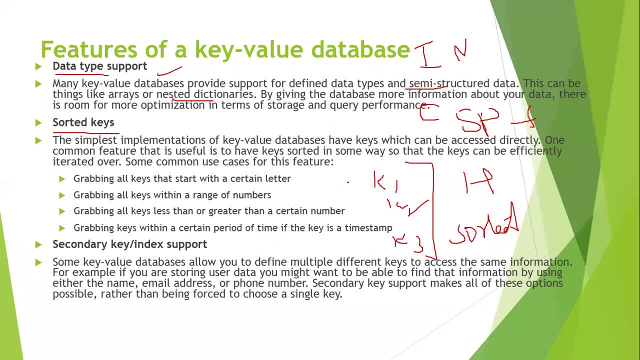 so this key stored database allows us to store the data in a order so that we can get the data very easily to the user right and secondary key and index support. so you know already the meaning of index. what is the use of index in your books? it will search the data very fastly. that means 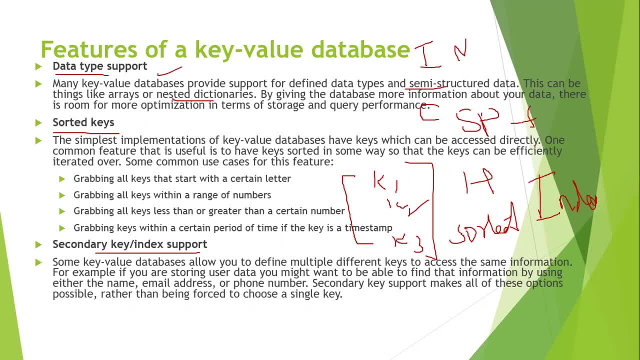 first index, after searching for example. third unit is: find it in the 104 page. so this is the key stored database allows us to store the data in a order. so we'll go to the 104 page and we'll read it from there, but that means by using the indexing. 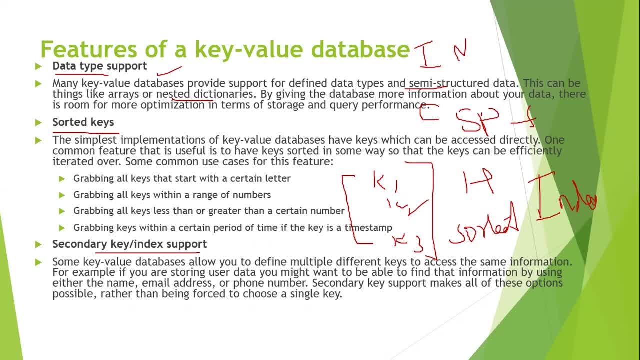 concept. we search the data very fastly, so this key value database allow you to define multiple different keys to access the same information. for example, if you're storing the user data, you might want to be able to find that information by using either name or email address, for example. 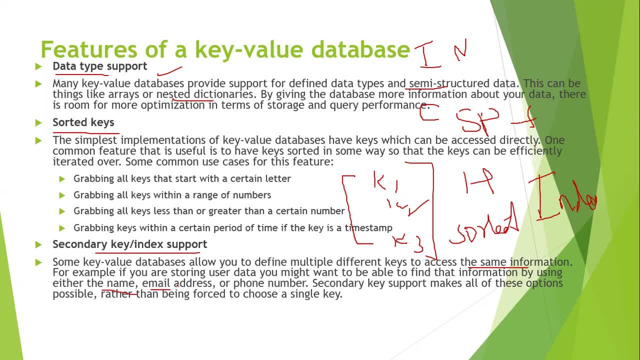 book: topic name: topic name: topic name. topic page name page name page. so only a topic name is not enough a word. for example, a page has 10 words in it. in those words we can take some words and prepare the index, not only taking topic name and page. 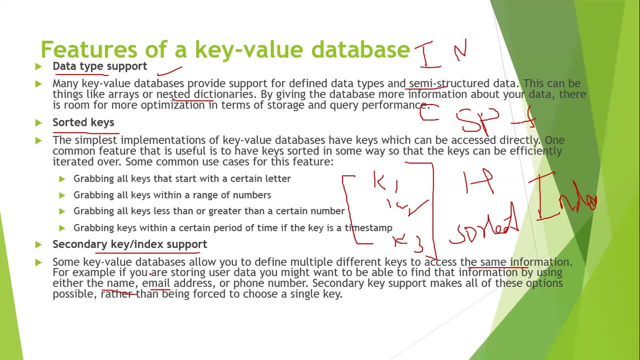 number. we can take few imported points from that and we can prepare a separate index for that imported points. so appendix will be there for the last key. so book meaning: what is that word? that particular page is going to be in the next page, so we can take a few words from that and we can. 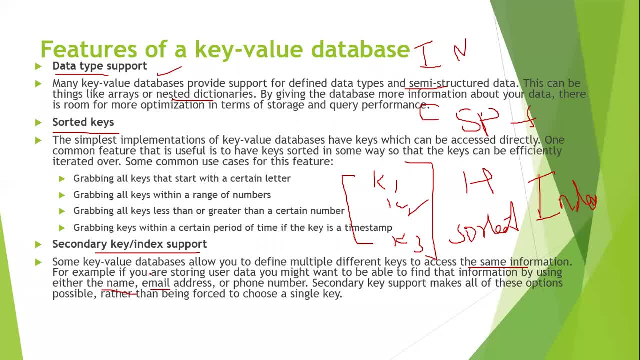 copy them all together to create a copy shirts. do they have there which texans are? when you enter the name, fit that. do you understand or not? by the way, giving Samsung and what's passed from association brief. actually it means it's very colour which is stuck and you can change it every time, which is 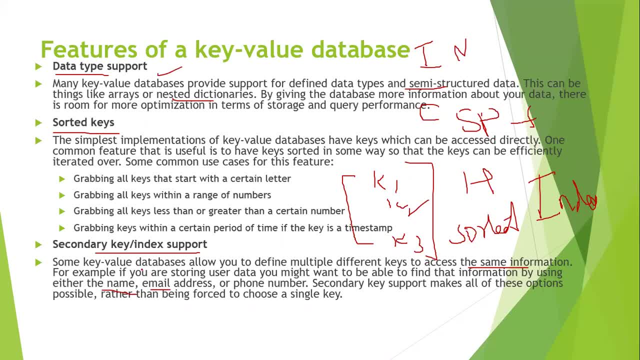 set like to complete the model, the index, where a lot of your necessary first things skill for visuality kına it for background beset codes so that can be escorted for using corporate. you will get a chance of getting three boxes into any celebrating fee and i thought that not only that, are just these disks in which i have. so underneath are the 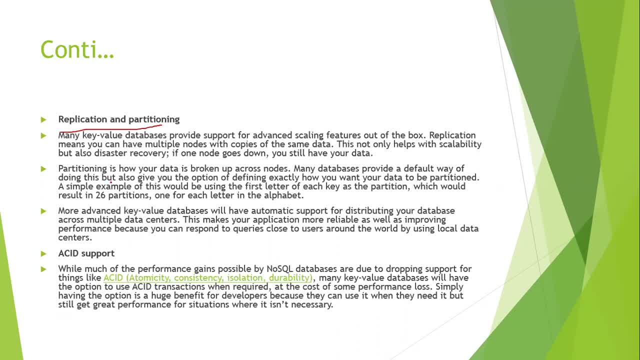 things you know. the by of data participation is nothing but participating how your data is broken up into different access nodes. many databases provides a default way doing this, but also gives you option to define exactly how you want your data to be participant, for example. consider an example here, first letter. 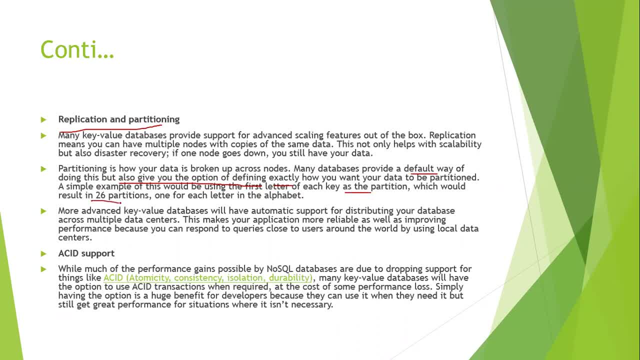 of each key participation, which would result in 26 partitions. one of each letter is in alphabet. for example, i want to define it as a. i want to define it as b, c, d, e, like this: i want to make it a partition. my database and more advanced key value database will have automatic support of. 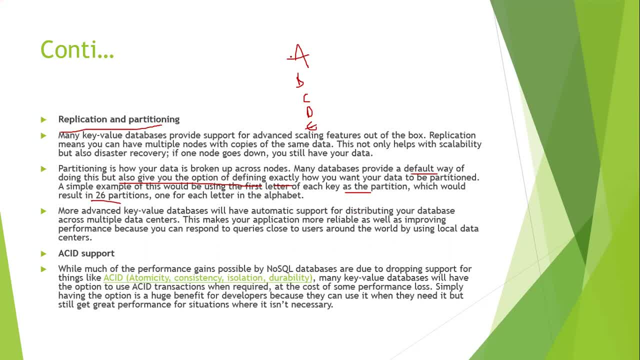 distributing your database across multiple data centers. that, in the sense, what? for example, i have database. in this database i have one lakh data, one lakh records i have. so this one lakh records if i'm storing at one location, if the day, if the particular database is one location, if the database is one location, if the database is. 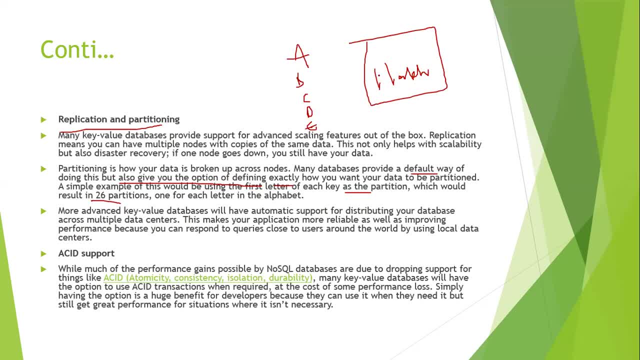 particular system is crashed, what happens? the data may be lost, but key value database also available in the cloud. so this one lakh database data is divided into some partitions and each partition is stored in a different system. so if you want to get the data first, you gather all the. 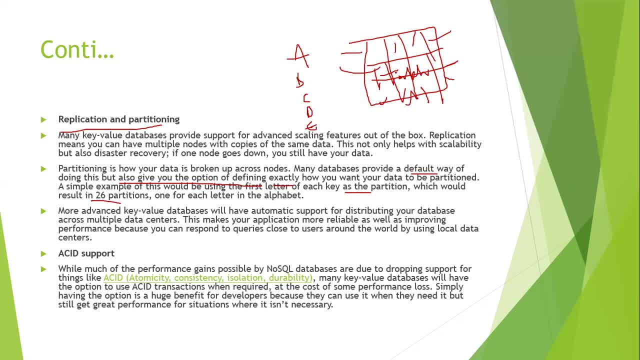 data and you do the modification again. you distribute the data. next, acid support. acid is nothing but atomicity, consistency, isolation and durability. so every database transaction should follow this acid property. so in later sessions we'll discuss about what is acid properties. if you are interested about acid properties, i have a youtube channel in that i have a video about this acid properties. 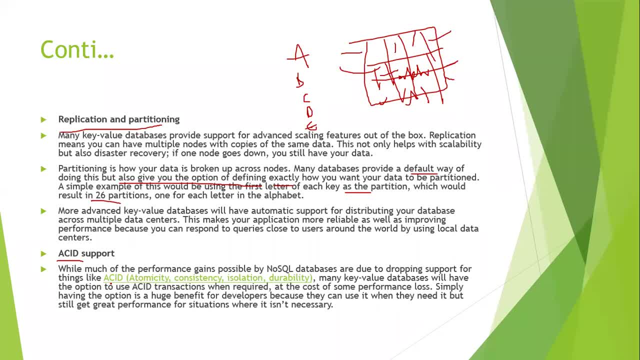 just grow through that acid properties. nothing but before transaction. for example, i'm debiting some amount from my account and i'm doing that, i'm sending that amount to my friend. so before that i have thousand rupees. if i send 10 rupees to my friend after that, what amount will be 990? 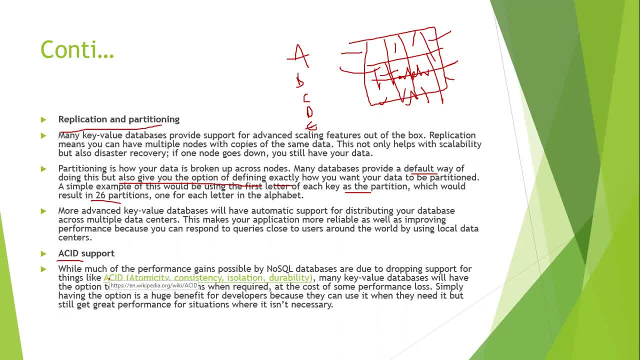 that means before transaction, your amount is right. after transaction, your amount is right. so then only the transaction is well and good and stored in the database. if the transaction is not done properly, then the data may be wrong. so consistency is not there in the database. but the key value database should support acid property. what the transactions you are doing. 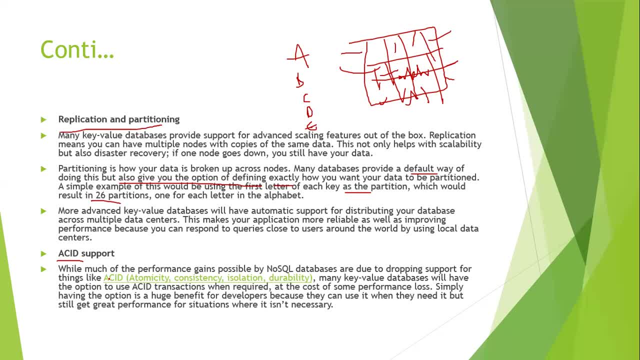 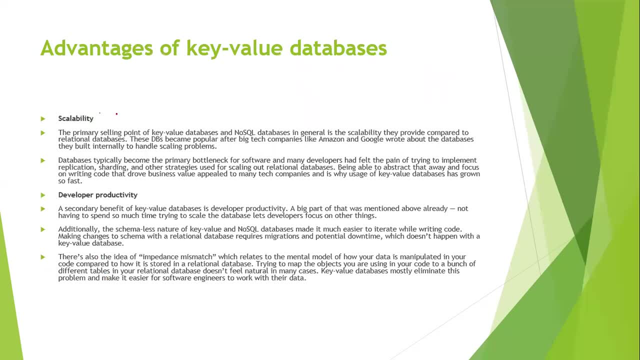 by using this key value database you are doing is not going to be used for the transaction. so, value database, all the data must be correct before and after transaction. and scalability. scalability in the sense what easily you can change the data in the database. next, developers: productivity. so developers will take the productivity in the sense if i'm, if i want to. 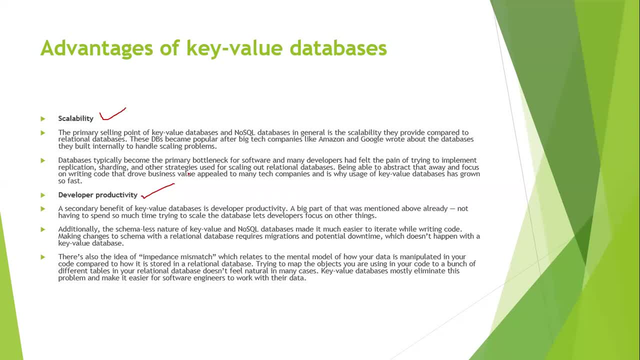 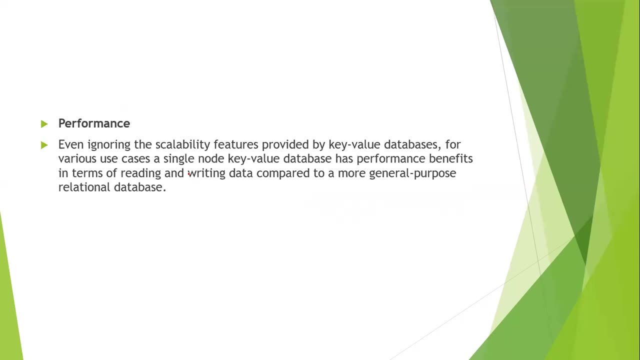 develop a database for my college. so i can develop the database for my college, i can develop my productivity in the sense developing a database for any organization is very easy and performance, so performance also very high in the key value database because it is a scalable, scalable means. 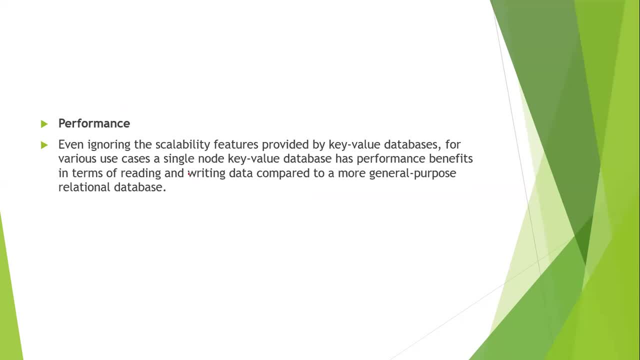 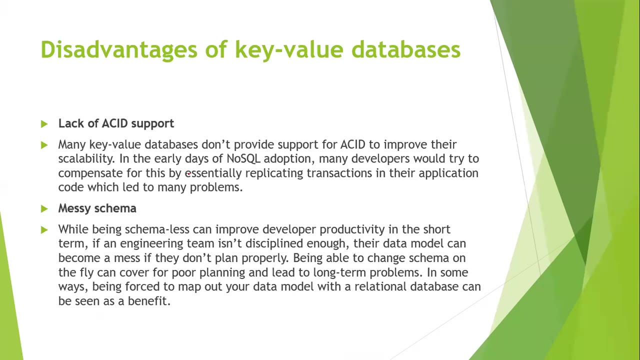 easy to modify, easy to understand, easy to write and reliable in the sense correct. so it is having more number of features. so in the market, everybody using key value database. so some of the drawbacks we have with the database. so lack of asset properties, so all asset properties are may not be satisfied with the 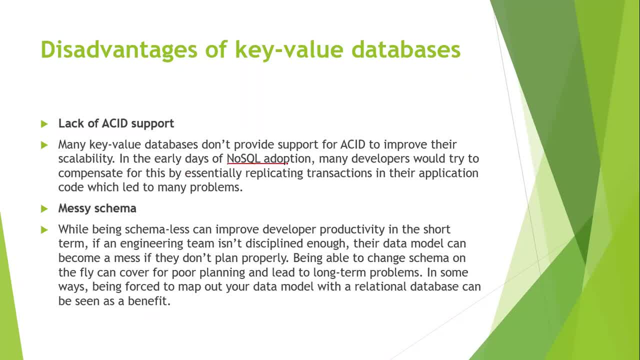 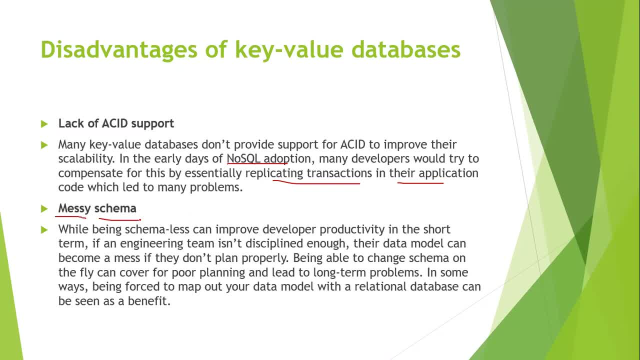 implemented in the key value databaseso many number of schemas can be implemented in the key value database. that means what? for example, if i want to find a route for a particular place, i can have any number of ways for that. similarly, in this also, while being schemaless can improve the developer productivity. 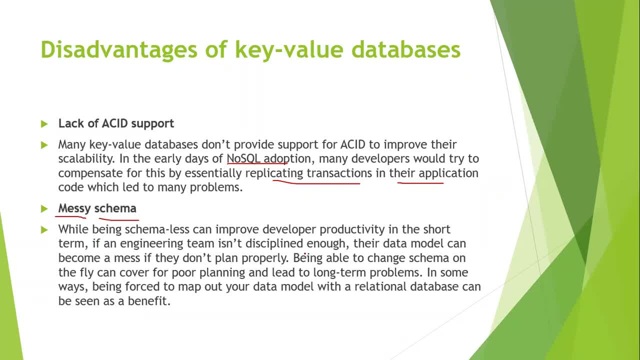 in short term. if an engineering team isn't disciplined enough, their data model can become a mess if they don't plan properly, being able planning and lead to long-term problems in some some ways being forced to map out your data model with the relational database can be seen as 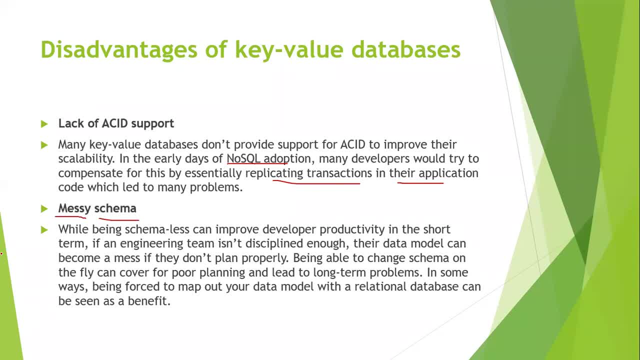 benefit. that means what mess? in the sense wrong schema is nothing but diagram. for example, if you want to construct a house first, what we do? we go to the architecture and we design a plan for that and we draw it on a paper. if the architecture is not designed, you are building. well, what is? 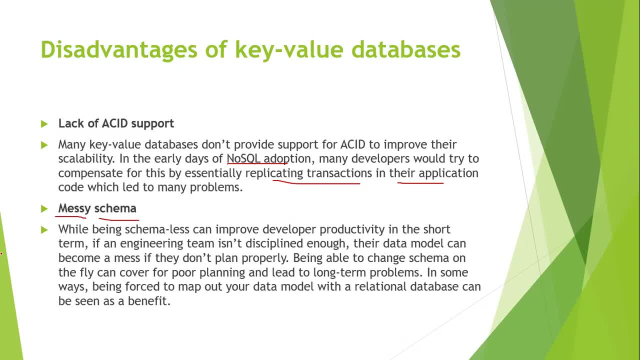 happening, your whole construction will be designed not properly and cannot be fit for our requirements. so here in the key value database also, if you are not designing properly, your data may mismatch, your data may loss, your made, your data may be incorrect and if you want to correct, 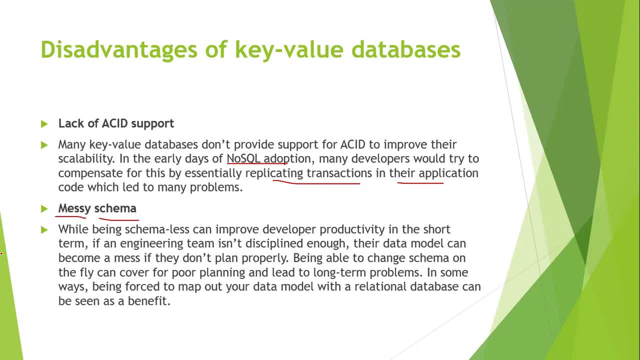 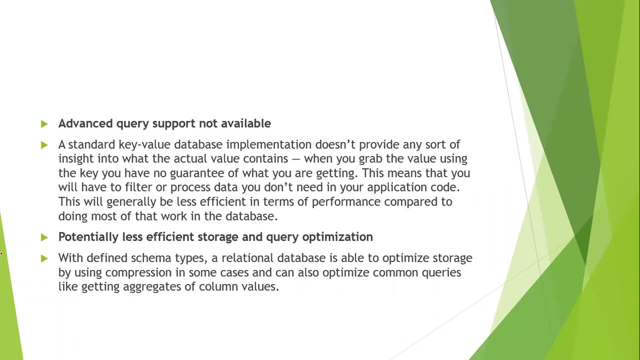 it. it may long time. that means whenever you are designing key value database you need to have more take care in the designing part. that is a one of the drawback of the key value database. advanced query support is not available. so sql is there. structured query language: so no, sql is also there, but it will. 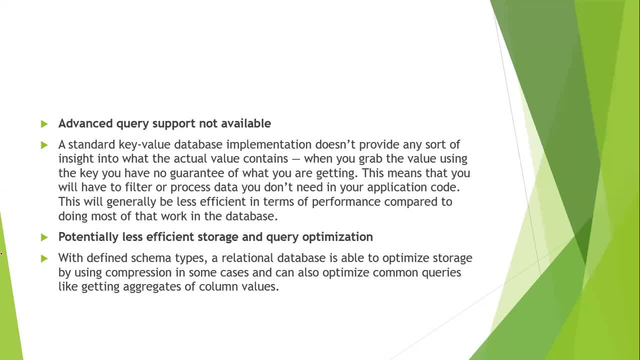 not support in advanced versions, potentially less efficient storage and query optimization. that means what: this key value database will not store large amount of data. if you want to store large amount of data, we go with mysql database. so this key value database will not have the capability of storing large amount of data and query. 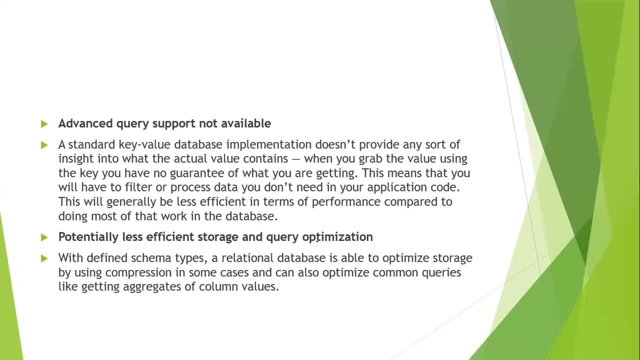 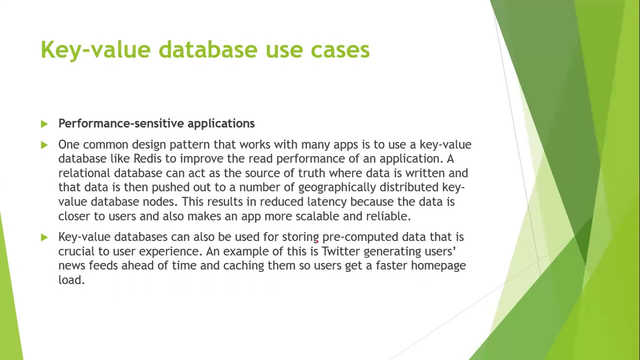 optimization query optimization in the sense, if you have a question, that question to be translated to the database understandable format. but this key value database is not having that amount of optimization techniques and performance sensitive, sensitive applications and this is suitable for only some reputed. that means some predefined applications will be there only. the performance will be there, available for the only. 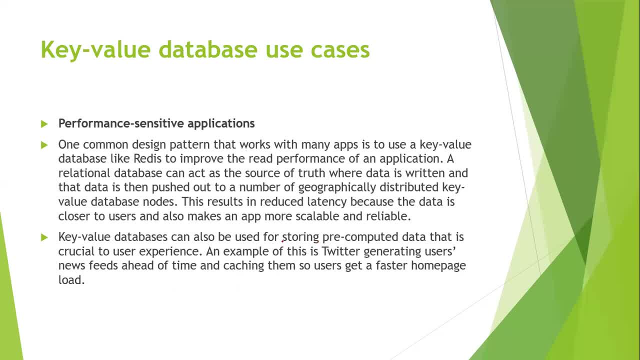 some of the apps are using this key value database. one common design pattern that works with many apps is to use key value database like ready to improve the read performance, and relational database can act as a source with the truth, where the data is written and the data is then. 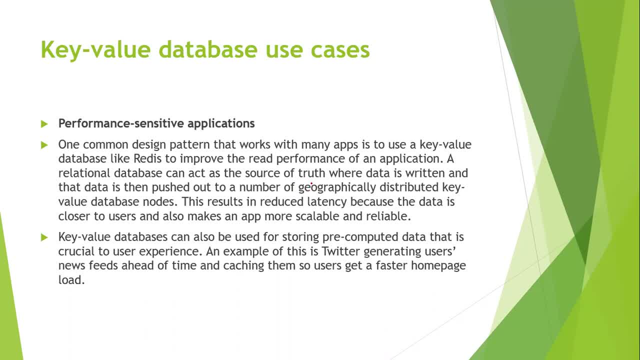 pushed to the number of geographically distributed key value database. this results in reduced latency, is more likely because the data is closer to the user and also makes an app more scalable and reliable. and clay applications because of the hashing- hashing or a concept of implementation and tough down to me compared to other type of databases. 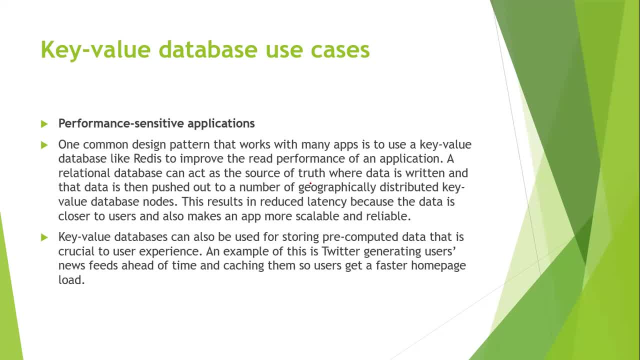 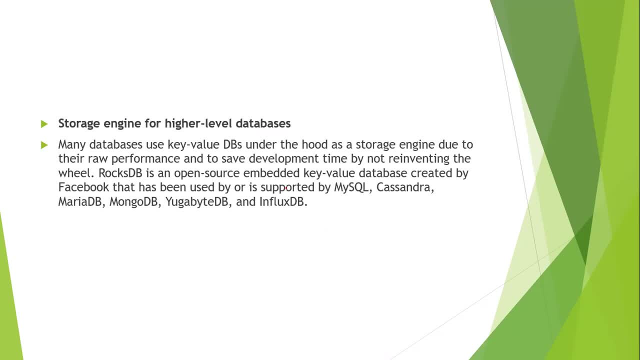 so on. the cause may only spider-minded key value database to use so strong engine for high level database. sorry, storage engine for high-level database. Many databases uses key-value database under the hood as a storage engine due to their raw performance and to save the development time. 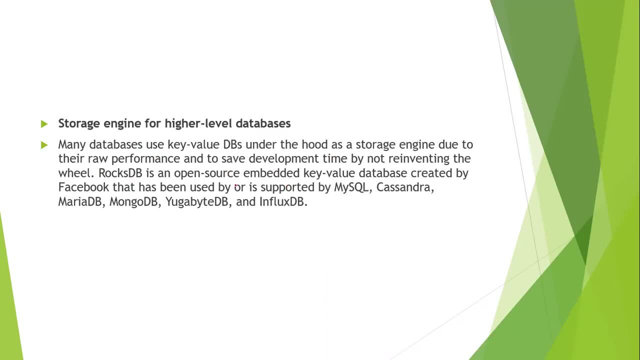 but not reinventing the wheel. RocksDB has an open-source embedded key-value database. So one of the key-value database is RockDB, created by Facebook. that has been used by, or is supported by, MySQL. So this MySQL is a very large database to have different kinds of databases. 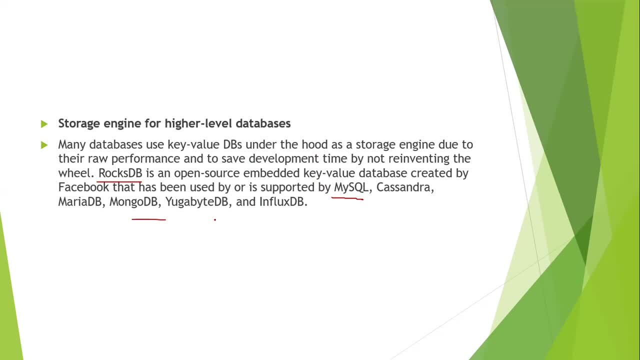 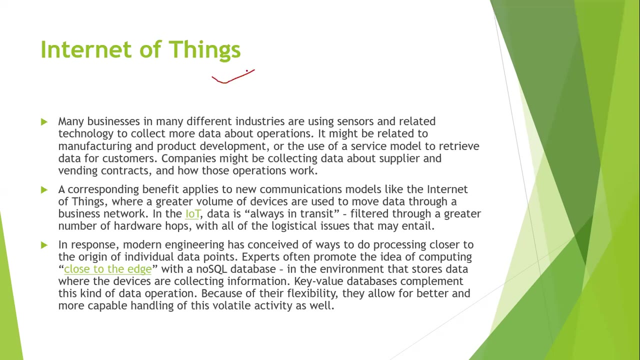 Now Cassandra, MarianDB, MongoDB and InfluxDB. all these are the different types of key-value databases which can be used by many number of organizations. So next Internet of Things. So in this Internet of Things also the key-value database is used mostly. 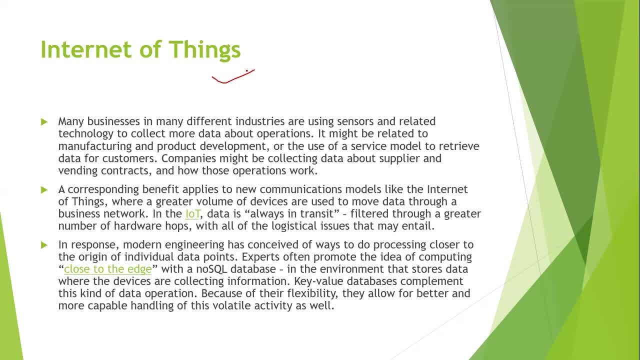 This is also one of the use case of the key-value database. This is also one of the use case of the key-value database. This is also one of the use case of the key-value database. 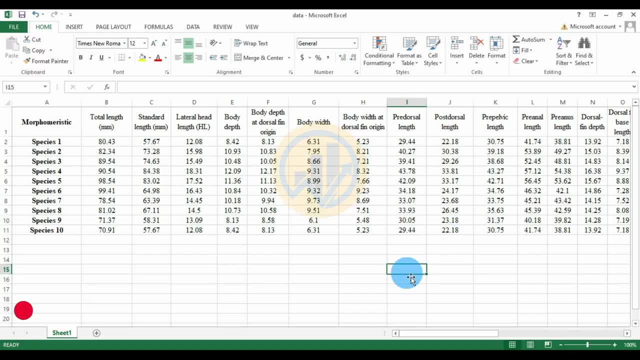 Hi everyone, welcome to statistics biosound youtube channel. Today we will discuss topic how to draw a two-way cluster analysis in past statistical software. The data already entered in the exercise sheet. The first: we take the 10 different species and the species morphometric parameters, the total length, the standard length and the dorsal gate and the body. 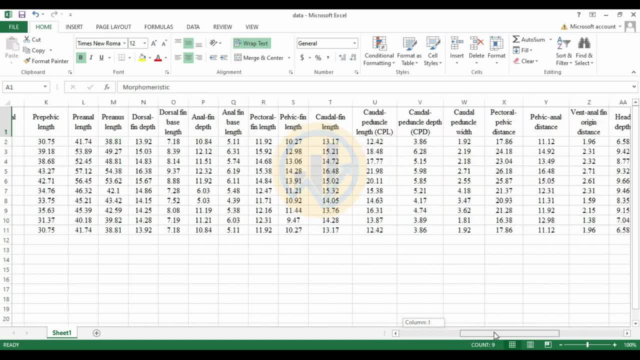 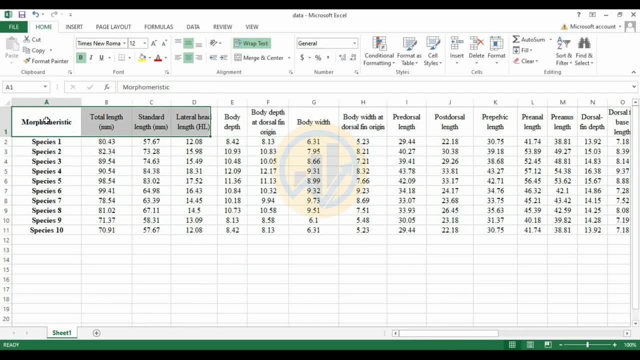 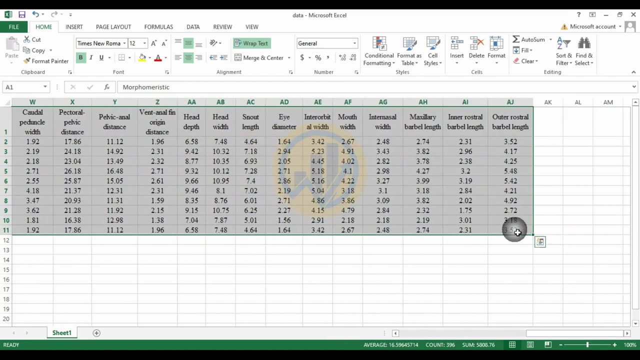 depth, also the morphometric parameter. for the different morphometric parameters. this data copy paste to the past statistical software. now the first copy the data, the copy the whole, the data. first select all the data under copy copy. go to the past statistical software, the. before we click. 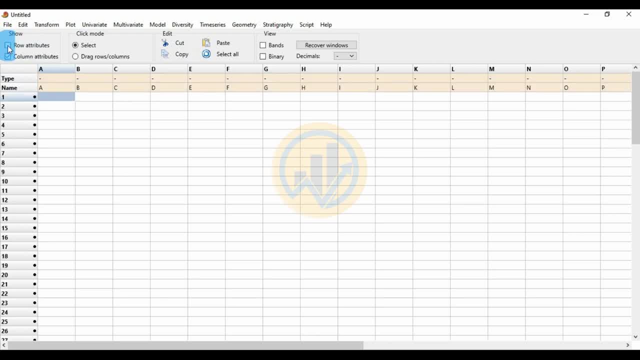 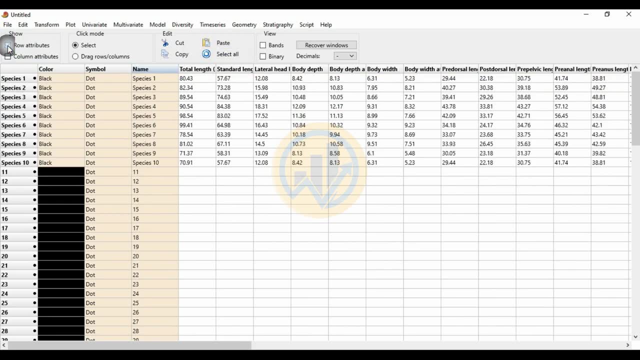 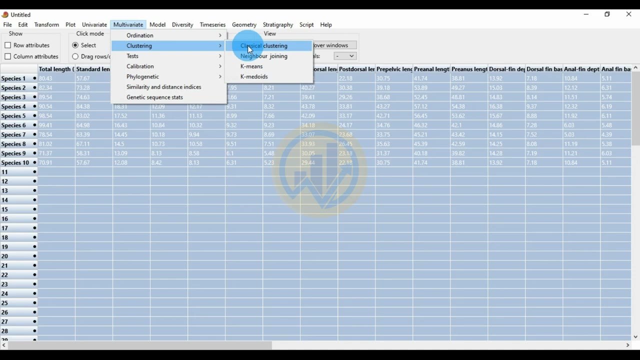 to the column attributed checkbox under the row attributed checkbox. then the paste the data. okay now. now the unclick the column attribute and row attribute and select the whole the data. go to the multi-varied menu under clustering and classic registering, the sub menu for clicking this graph. 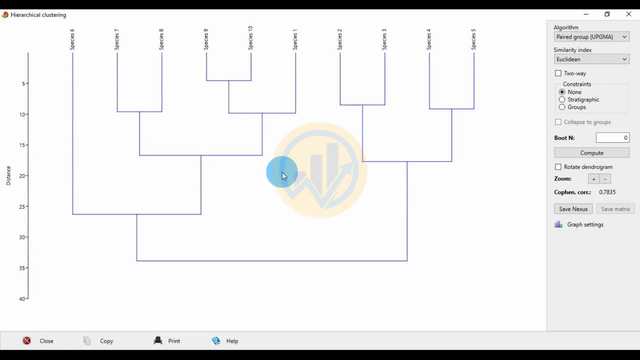 okay, open the new tab for the clustering analysis in the species, the 10 different species, the algorithm for the pad group, upgma and the similarity index for the change to the bi-ray cluster. now they click the computer, they change the bi-ray clusters. this is a bi-ray cluster, the